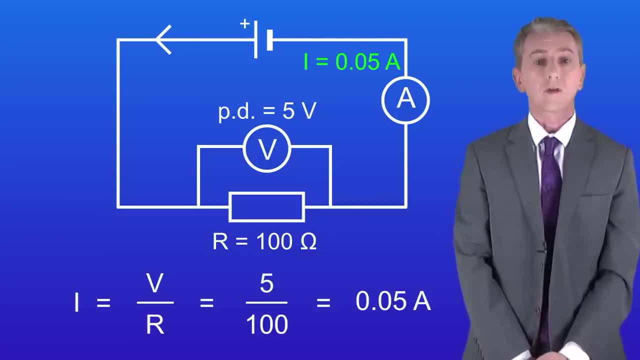 hundred ohms. Putting these into the equation gives us a current flowing in the circuit of 0.05 amperes. Now in this video we're looking at circuits which contain more than one resistor. Let's start by looking at resistors in series. Take a look at this circuit. 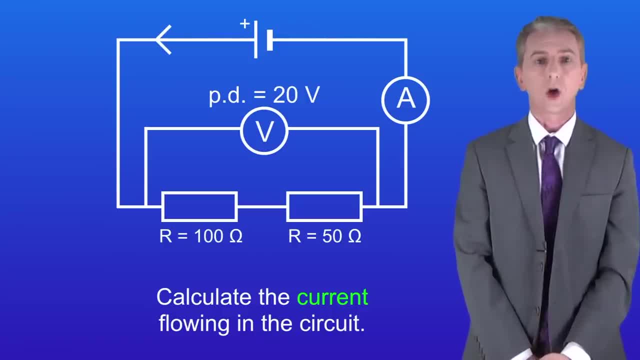 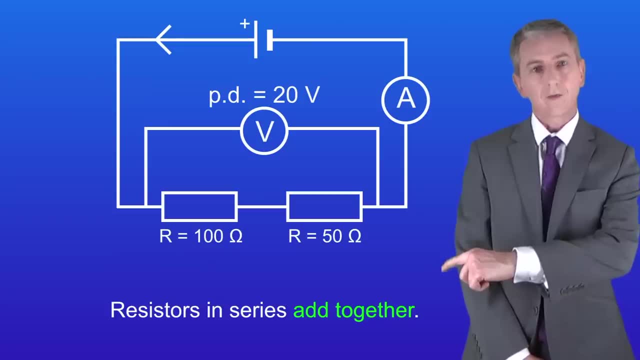 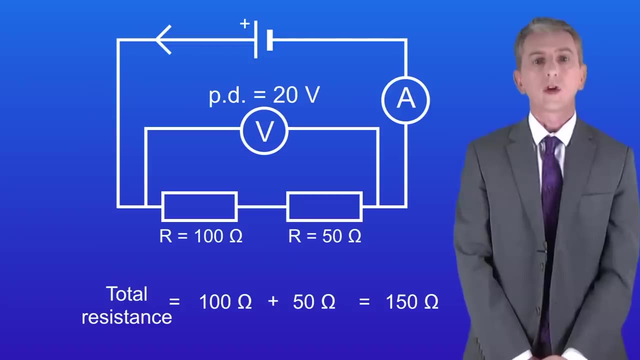 Here we've got a 100 ohm resistor in series with a 50 ohm resistor. The potential difference is 20 volts and we've got to calculate the current. So here is the key factor you need to look at: Resistors in series add together In our circuit. we've got a 100 ohm resistor and a 50 ohm resistor. 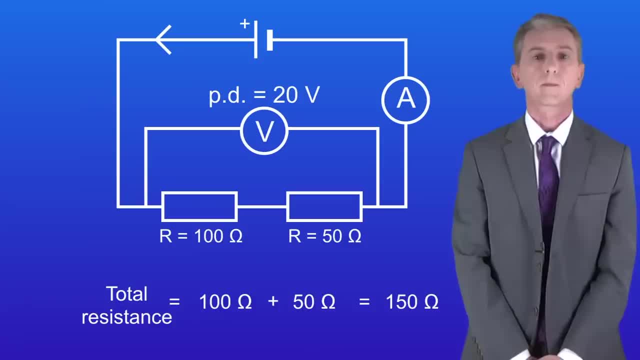 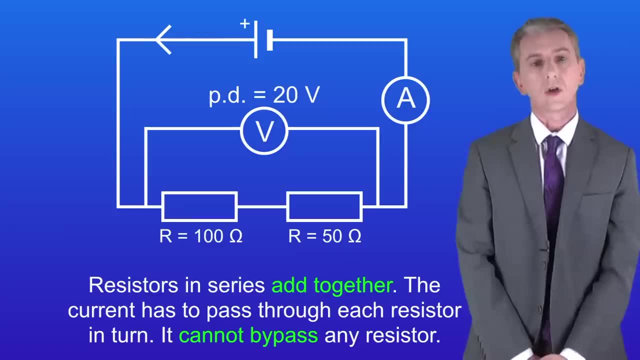 So the total resistance is 150 ohms. Now it makes sense that resistors add in series. That's because the current has to pass through each resistor in turn. It cannot bypass any resistor. What that means is that we could replace these two resistors with one 150 ohm resistor, like 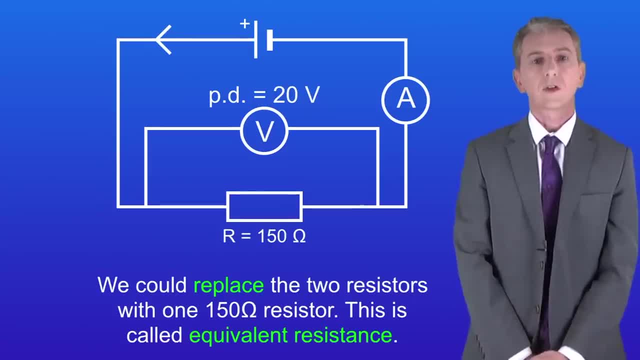 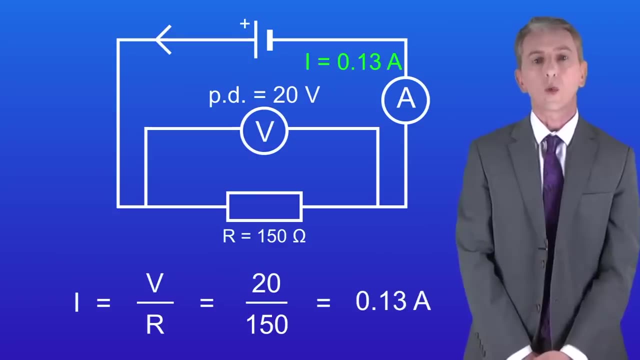 this. Scientists call this equivalent resistance. Going back to our equation, we can now calculate the current in this circuit. The potential difference is 20 volts and the combined resistance is 150 ohms. Putting these into the equation gives us a current of 0.13 amperes. 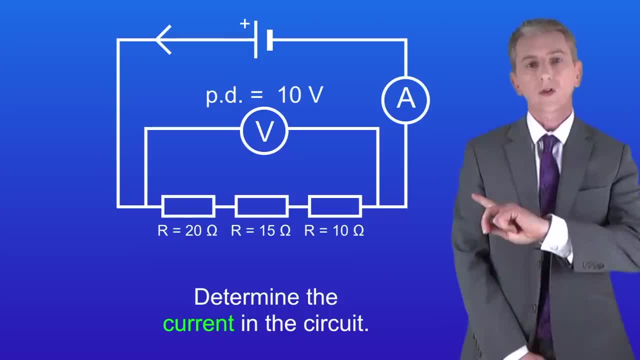 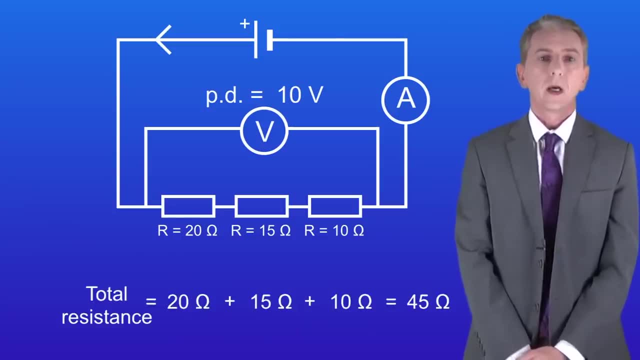 to two decimal places. Here's a question for you: Determine the current in the circuit. Pause the video and try this yourself. Okay, we've got a 20 ohm resistor, a 15 ohm resistor and a 10 ohm resistor, all in series. Adding these: 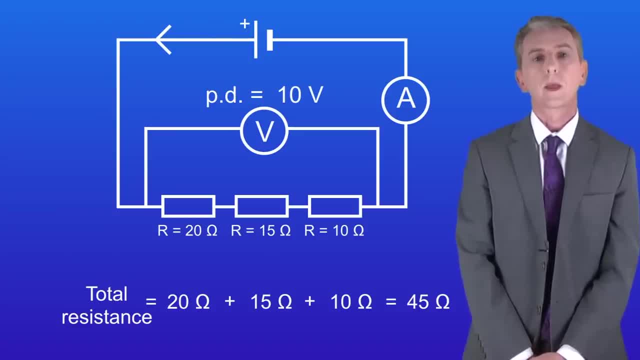 together gives us a total resistance of 45 ohms. The potential difference across these resistors is 10 volts. We can calculate the current by dividing the potential difference by the total resistance. So 10 divided by 45 gives a current of 0.22 amperes to two decimal places. 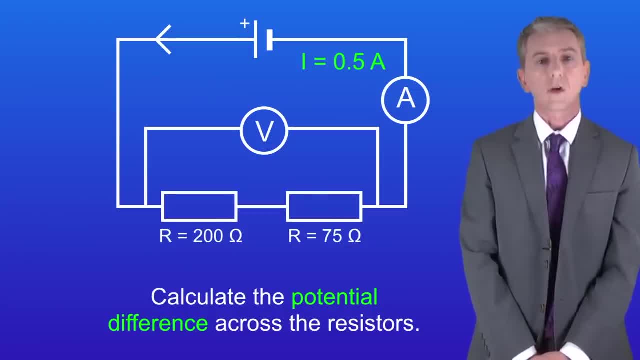 Here's another question for you: Calculate the potential difference across the resistors. Pause the video and try this yourself. Okay, so first we've got to calculate the total resistance. 200 ohms plus 75 ohms gives a total resistance of 275 ohms.